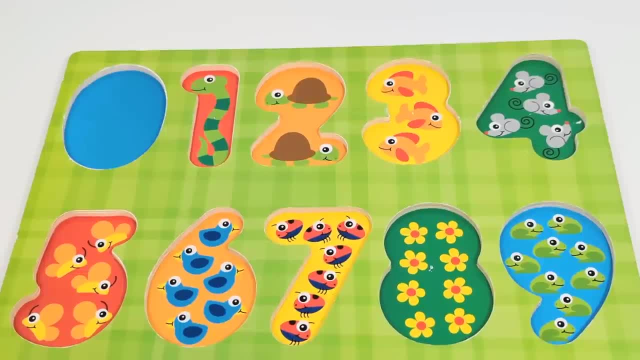 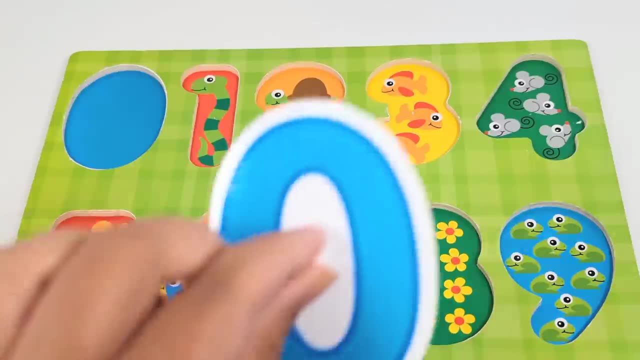 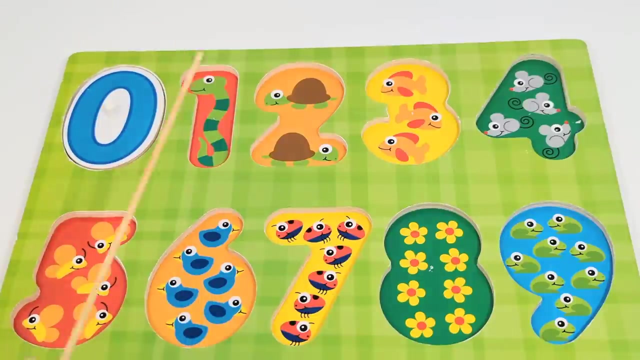 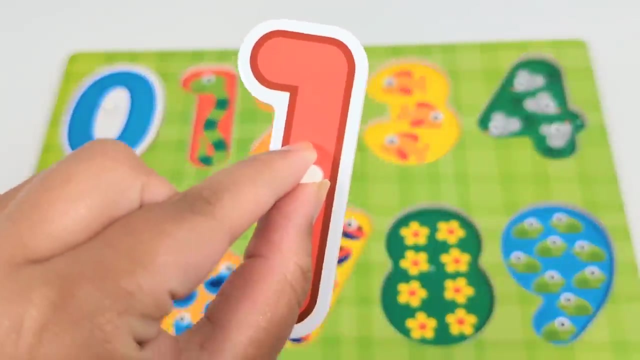 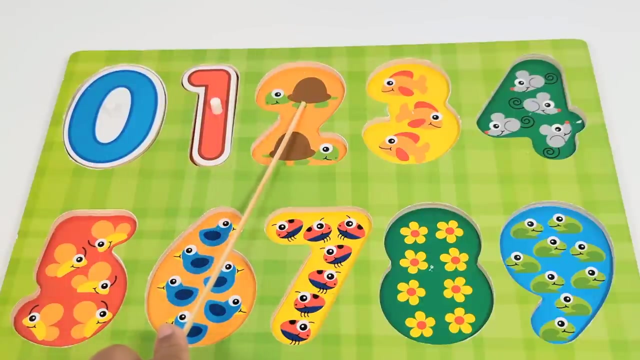 Hey, activity learners. Today we're going to learn and practice our numbers using this number puzzle. The first number is zero, Zero. The next number is the number one. There is one snake, One, One. The next number is the number two. There are two turtles. Let's count One, Two. Number two. 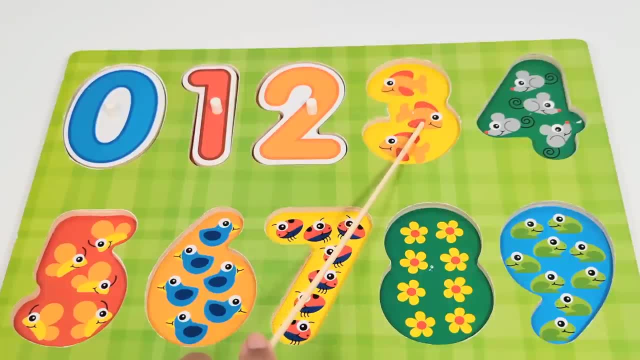 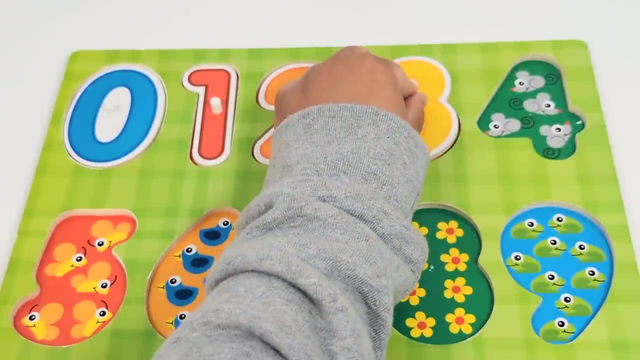 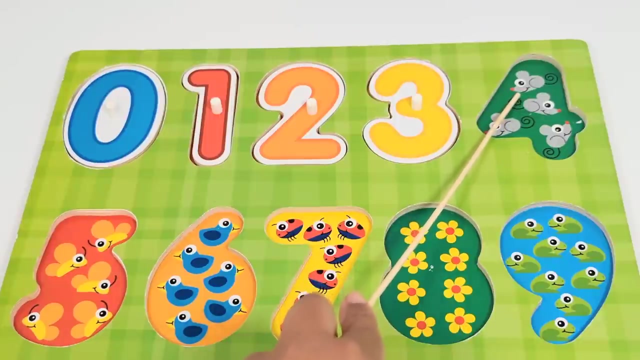 The next number is the number three. There are three fish. Let's count One, Two, Three, Number three. The next number is the number four. There are four mice: Let's count One, Two, Three, Four, Number four. The next number is the number five. There are five turtles: Let's count One, Two. 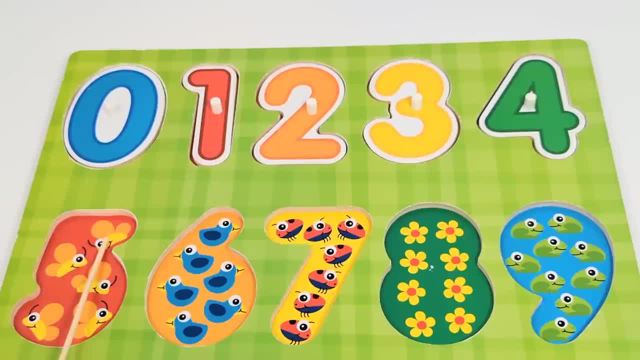 Five butterflies. Let's count One, Two, Three, Four, Five, Number five. The next number is the number six. There are six birds. Let's count One, Two, Three, Four, Five, Six, Number six. There are six birds. Let's count One, Two, Three, Four, Five, Six. 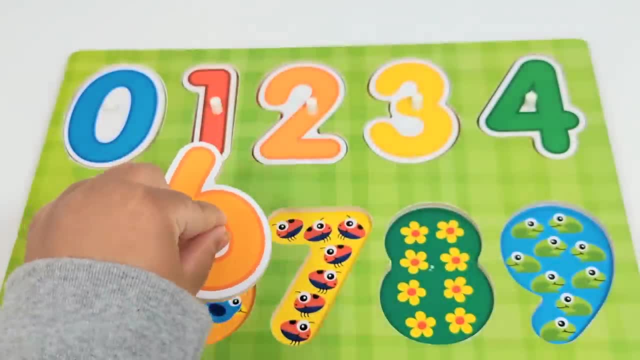 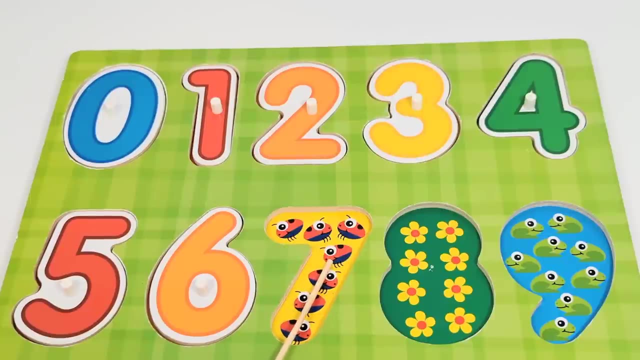 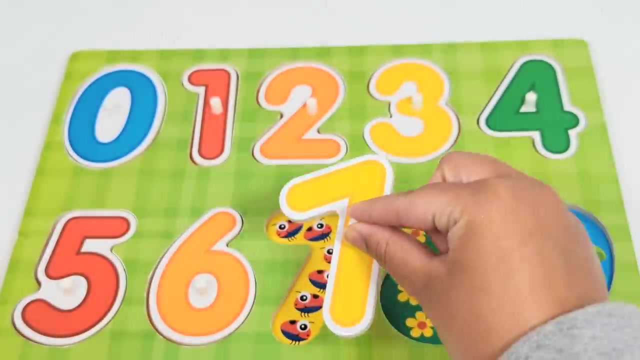 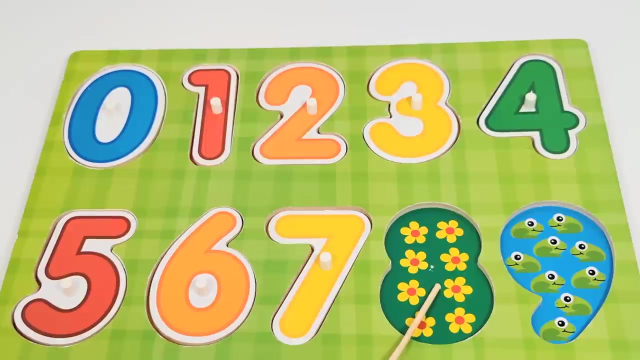 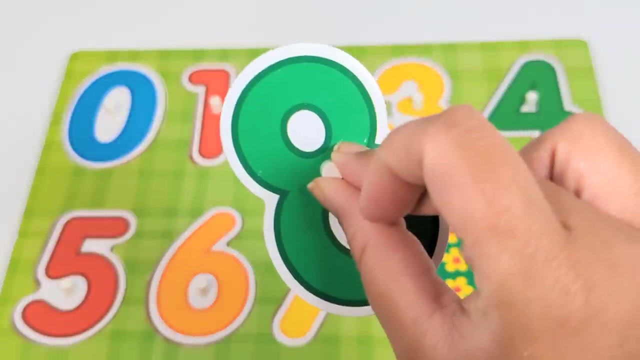 Number six. The next number is the number seven. There are seven ladybugs. Let's count One, Two, Three, Four, Five, Six, Seven. Number seven: The next number is the number eight. Number seven. The next number is the number eight. There are eight flowers. Let's count One, Two, Three, Four, Five, Six, Seven, Eight.